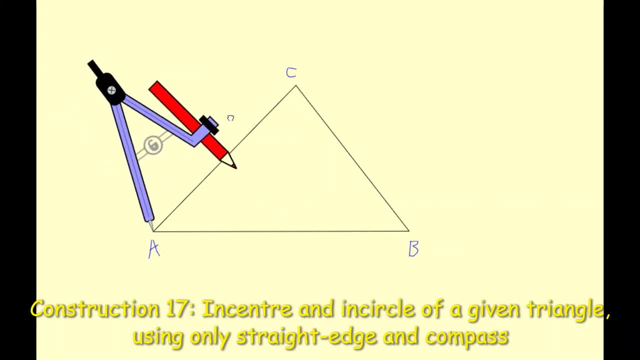 the pencil. it doesn't matter if you go beyond halfway, So make it a distance that you're comfortable with. I'm just going to approximately halfway. Just make sure that the radius you pick for one side must be consistent throughout the whole question. I'm then going to draw. 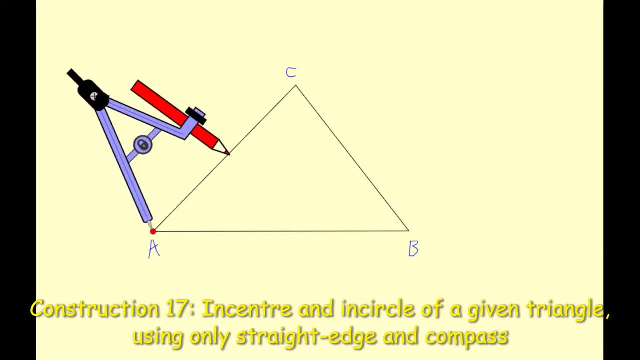 an arc on this line, segment AC, And then I'm going to bring my compass down and I'm going to draw the arc on the line AB as well. Now I'm going to move the nib of my compass to both of these arcs And, once again, I'm 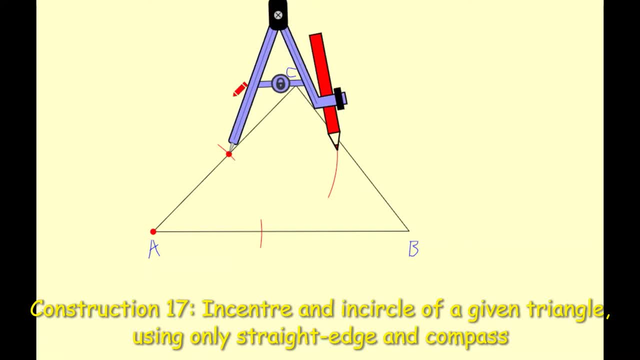 going to draw two arcs, And the two arcs that I draw at this time will hopefully intersect. So again, I never changed the radius of my compass And I'm now going to intersect my line. So that's the first arc. I put away my compass and now I'm going to use my ruler to connect. 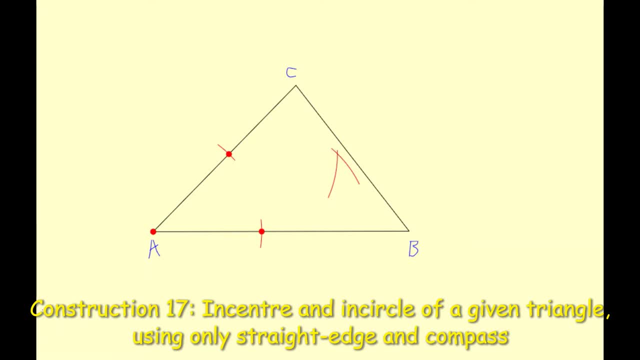 A to where these two arcs are intersecting. So sliding my ruler up to A and you can see it's crossing the two arcs and I'm going to connect that with my pencil. Again, I don't have to stop at the arcs, I'm going to carry. 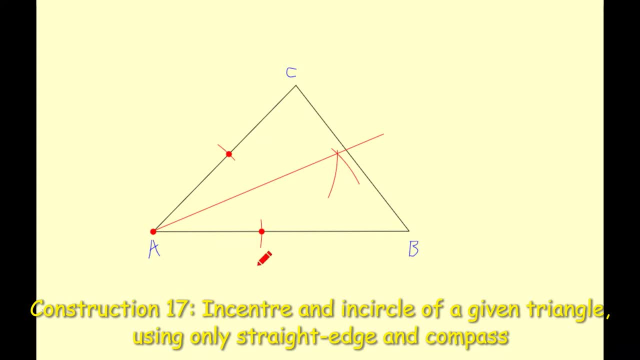 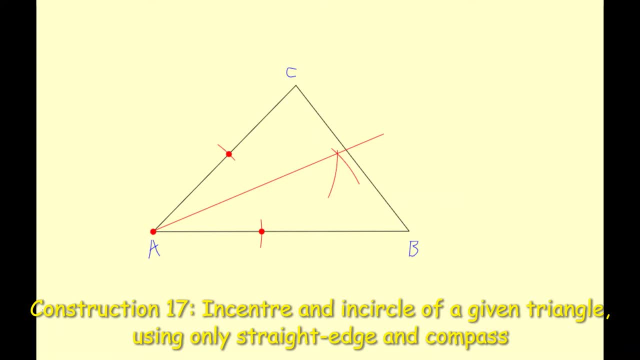 So I'm going to go from C to B, So I'm going to once again construct the bisector of the angle B this time. So I'm going to take out my compass and I'm now going to move it to the corner of B And I'm 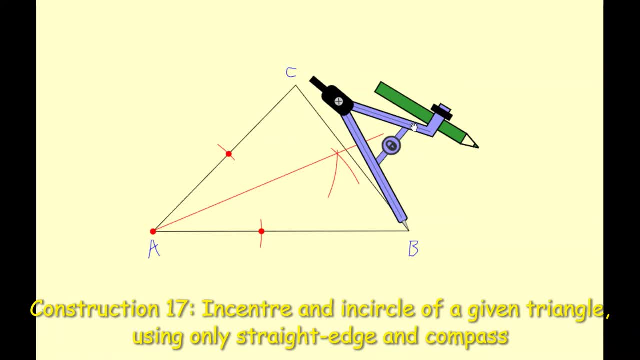 going to bisect the line CB and AB. So that's my first arc, and then I'm going to bring it down to B. So that's my first arc, and then I'm going to bring it down to B. So that's my first arc, and then I'm going to bring it down to B. 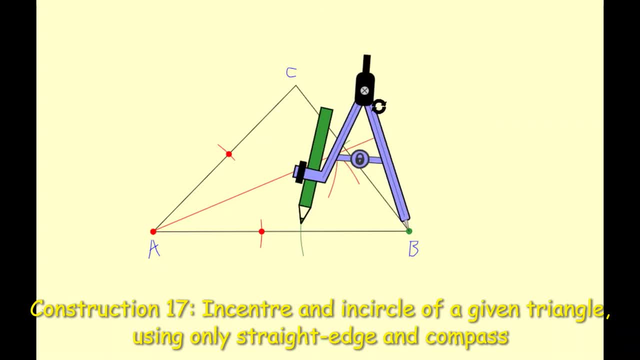 So there it is. So I'm BR skidding the compass pass to them a little bit and once again my sinter hurts and I'm going to be able to circulate the line every set, so to put in this there. so I just need to maybe bring the name of my compass back up and make sure. 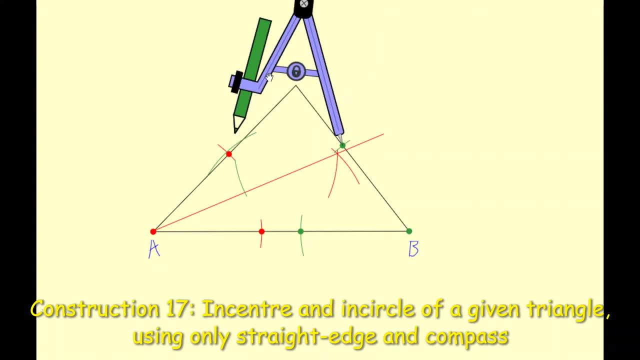 that I extend my arc far enough. so you can see here I just need to extend it ever so slightly. so that's what will happen in practice. sometimes you just need to come back and check your arcs. so I'm going to put away my compass and now. 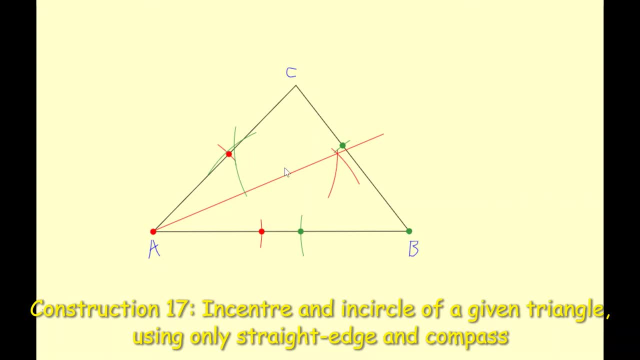 I'm going to take out my ruler and I'm going to draw a line from B to where these two arcs are intersecting, so sliding my ruler up to the point B. make sure, then, that it goes through my two arcs, which it does, and I'm going to 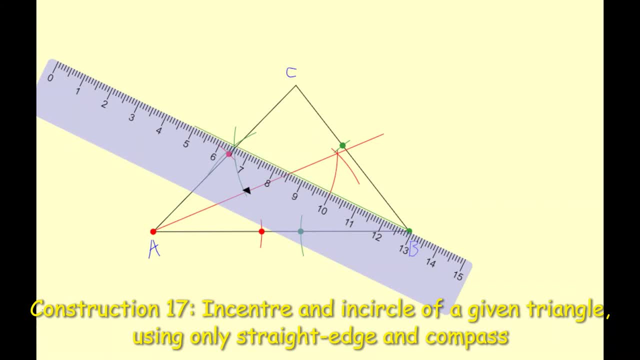 connect that now with my green line, and there is my bisector of the angle B. I don't need to carry out the bisector of angle C. you can if you want, but you will see that it will also intersect at the same point here. so I'm going to put a. 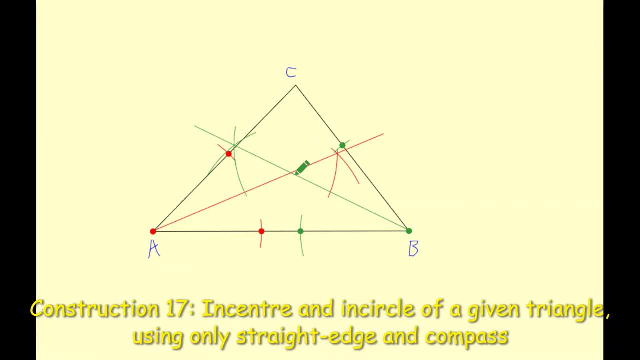 dot here where the green line and red line intersect, and that is what's known as the in-center. from my center I'm now going to construct the in circle and the circle is going to be within the triangle. so it's the in circle. so I'm going to put the nib of my 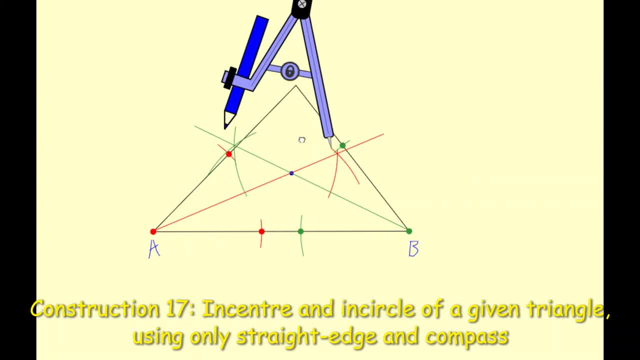 compass now at the in center. I'm going to reduce my radius of my compass now. this is going to touch the edge of my triangle, so it's touching it about here. doesn't matter if I went to the bottom or to the right hand side, I've just gone. 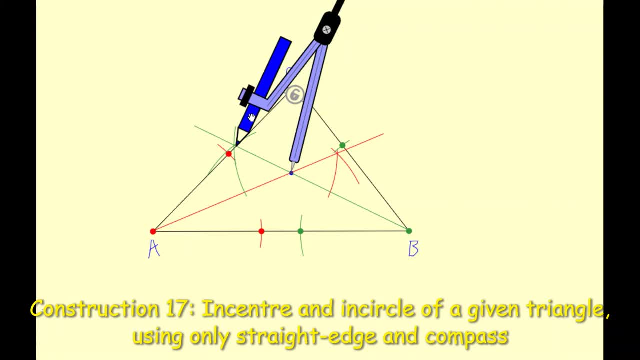 to the left. so just make sure that it touches the edge of the circle or of the triangle. I'm now going to hopefully rotate my compass and it should create a circle within this triangle, touching the three line segments. so let's see how we get on. so, fingers crossed, and I'm going to hold the Compass from the top. I'm